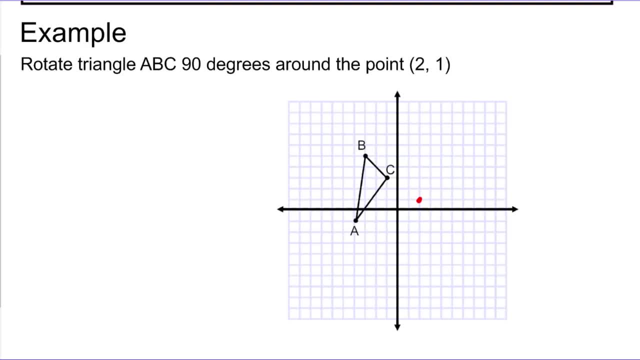 And so what that means is that the circle. let me get my little circle tool here. my circle is actually now centered. It's centered right here, and I'm going to travel around this circle in some way, So these points are going to travel around this circle instead of traveling around the original one. 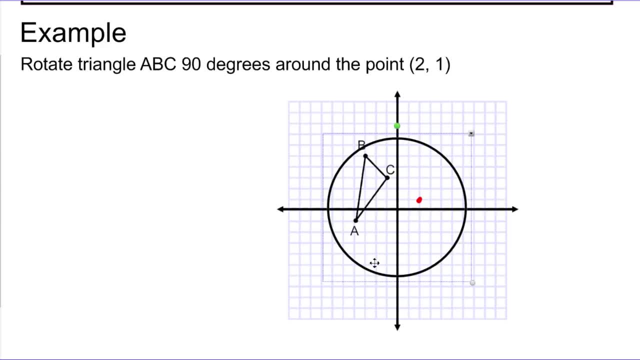 which was kind of centered over here at the origin. So by changing my center of rotation, I'm actually changing the circle that they're traveling around. Okay, and so here's what we're going to do. Let's pull our points off of the graph so we know what we're working with. 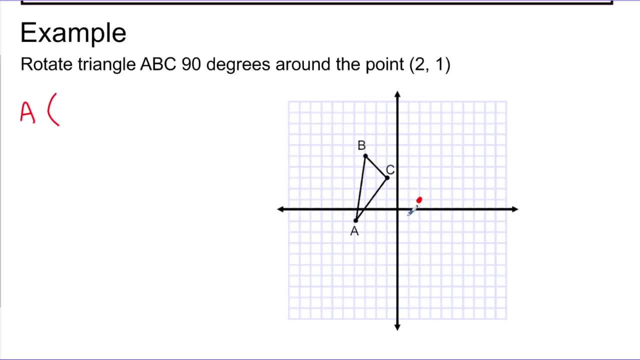 It looks like I have an a value okay of negative 1,, 2,, 3,, 4, negative 4, negative 1, okay, I have a b value okay. oh, let me get myself some space here. 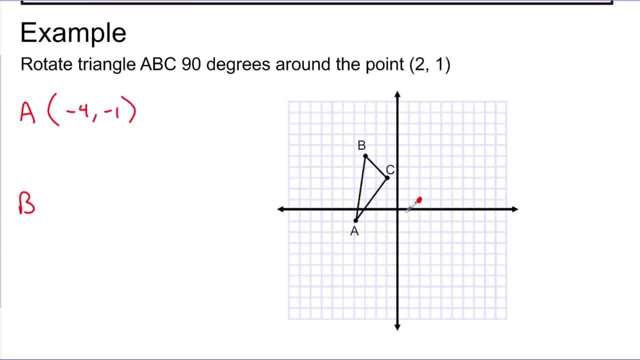 We're going to need a little bit of space, okay. b value of negative 3 and up to 1,, 2, 3,, 4, 5, negative 3, 5,. okay, and I have a c value of it looks like negative 1, 3, negative 1,, positive 3, right. 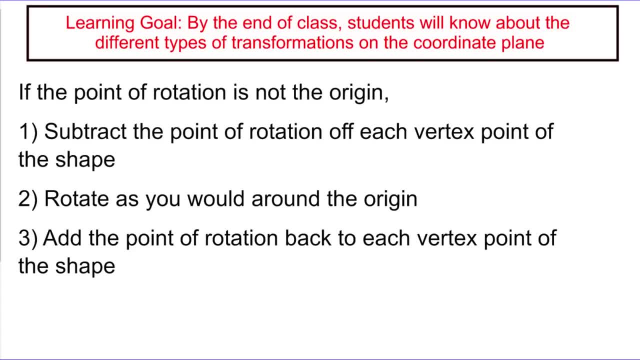 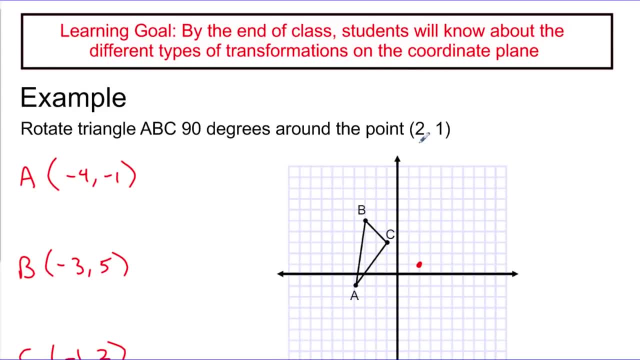 So what our rule here said was: if we want to rotate this, let's subtract the point of rotation off of each vertex. Let's start with that. So my point of rotation is 2, 1.. So they're asking us to subtract 2 and subtract 1 from each of these points. 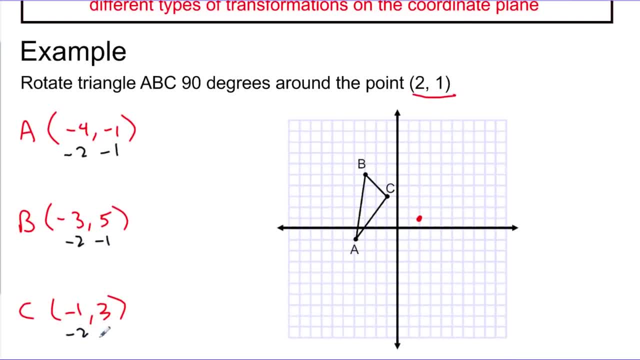 and what that's doing is it's kind of shifting the entire graph over two units- I'm sorry, over two units- to the left and down one unit which is going to move my center of rotation to the origin. So here's why, kind of like interim point- I'm not even going to call it a prime because it's not a prime yet- 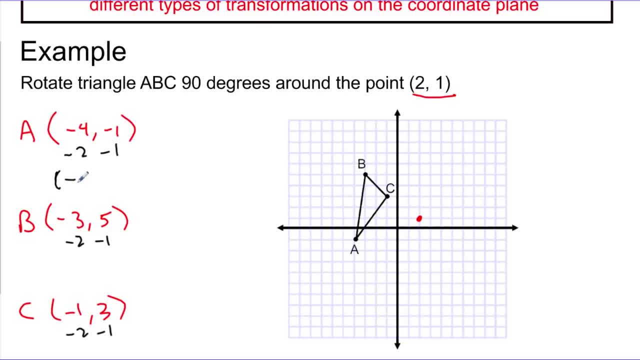 We haven't done our rotation yet. So if I do negative 4 minus 2, I get negative 6.. Negative 1 minus 1, I get negative 2, okay, And then I'm going to do that for each of these points. 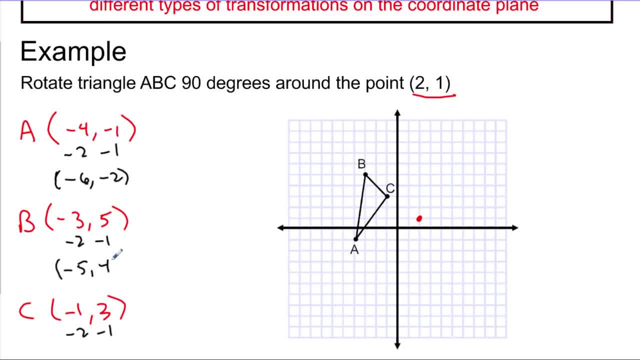 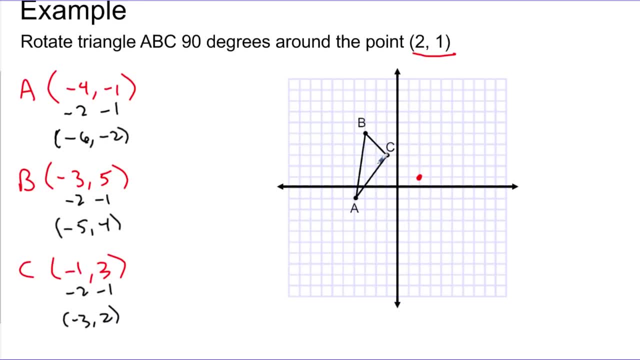 It looks like I get an interim point of negative 5, 4, and my c is going to go from go to negative 3, 2, right. So again, that's just kind of taking all these points and sliding them to the left by 2 and down by 1. 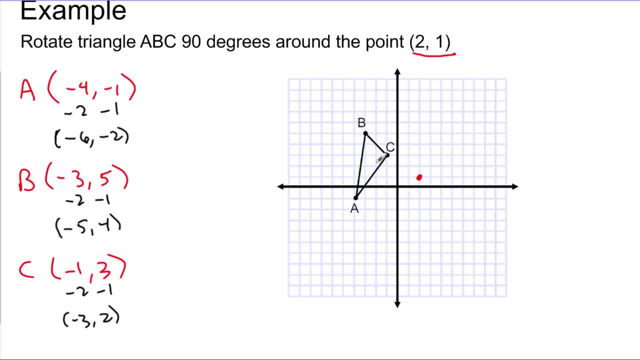 so that my center of origin- I'm sorry, my center of rotation can be at the origin. So we're going to perform our rotation, We're going to do the algorithm on these points here, these ones that I've slid over and down, okay, 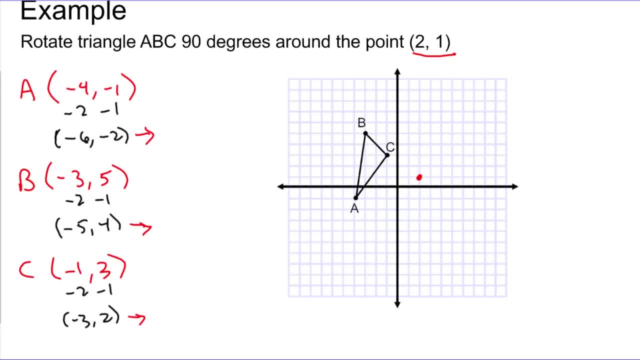 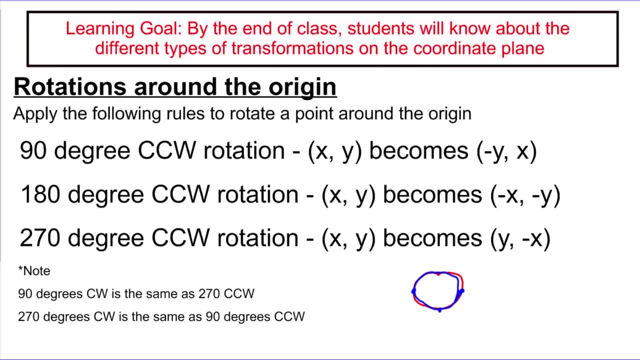 So if you remember the rule again that we had for a 90-degree turn, a 90-degree rotation here, it is okay. A 90-degree rotation is going to be a switch of the sine of y and then swap the x and the y values. 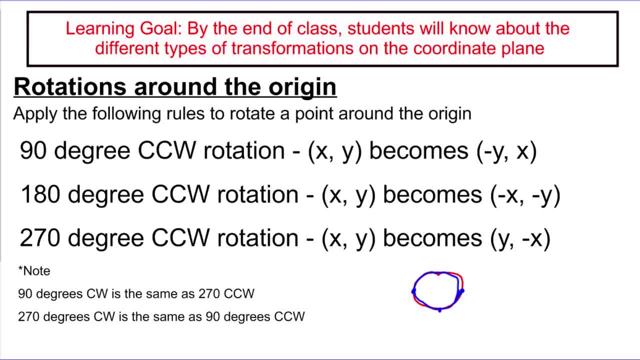 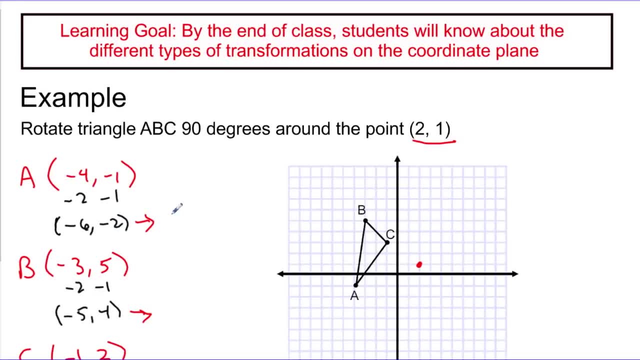 So that's the algorithm that we're going to apply, that we can apply now, because now my center is at the origin, So I'm going to switch the sine of y, which would make this positive. okay, So this one I'm going to call. I'm going to call it a, okay. 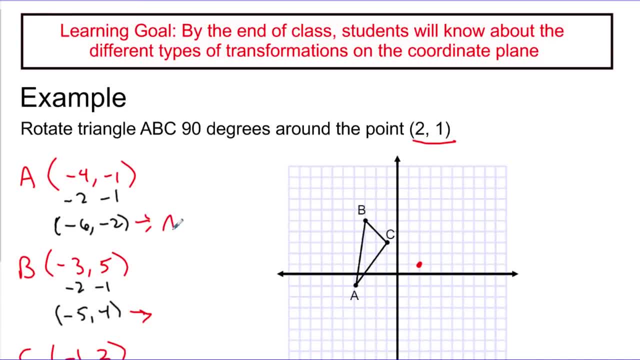 Call that a prime, okay. So I'm going to say my a prime is going to be positive 2, okay. Negative 6, okay. Oh, actually, you know what? I'm not going to call this a prime yet. 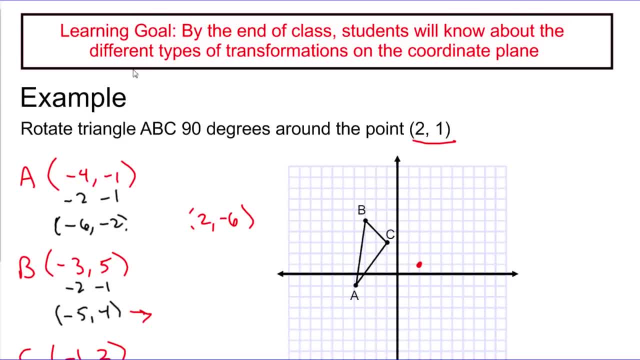 We have one more step left to do, so let me get rid of that, okay. So this is kind of another interim step, okay, where I'm going to take my point and do the rotation, okay. So I did my algorithm where I switched x and y and then flipped. 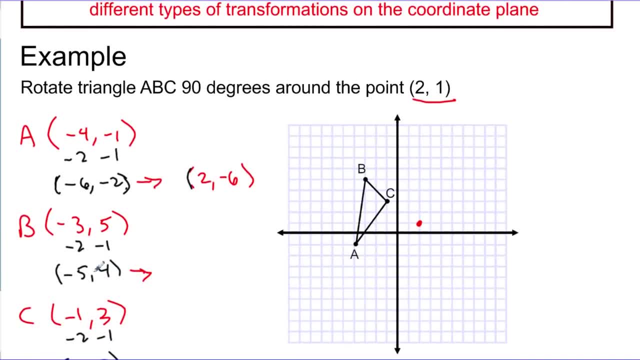 Let's do it again on this new b value Switch x and y after I've changed the sine of y. So this is going to become negative 4, negative 5, right, And I have one more rotation left to do. This is going to become negative 2, negative 3, okay. 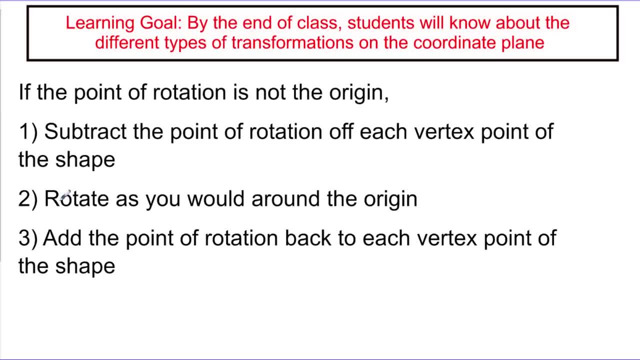 So now to get back to my final step here. So that was my rotation as we would around the origin. I used my 90-degree rule and I rotated around the origin. But now I've got to move all my points. Now I've got to move all my points back. okay, 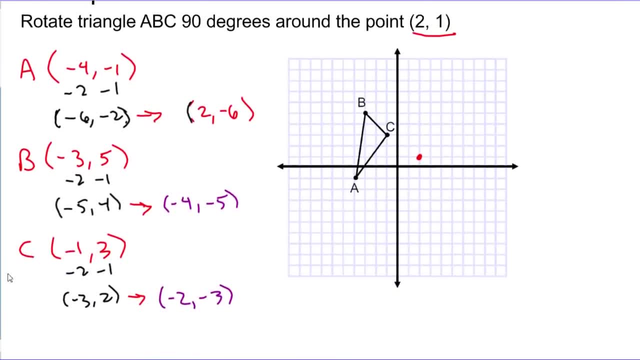 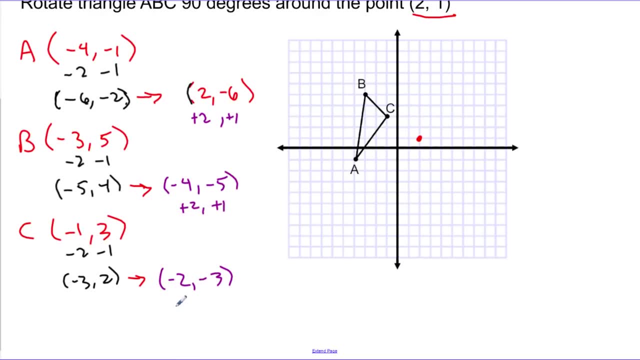 So I'm going to add in that 2 and that 1 that I took away at the beginning. So let's add 2 and add 1 to each of these points. Plus 2, plus 1, plus 2, plus 1, right. 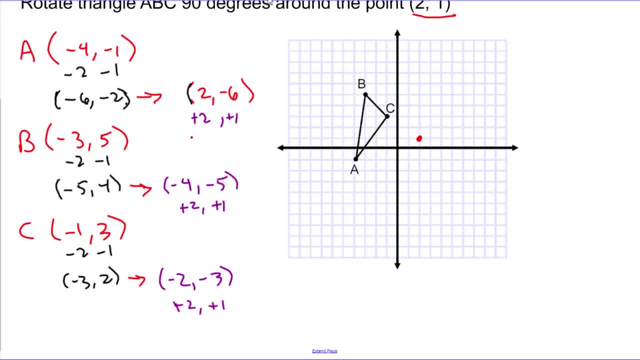 So now here's my final rotated points. This, which I'm going to use another color here, this is my a prime. This looks like 4 and negative 5, okay, This one looks like negative 2, negative 4.. 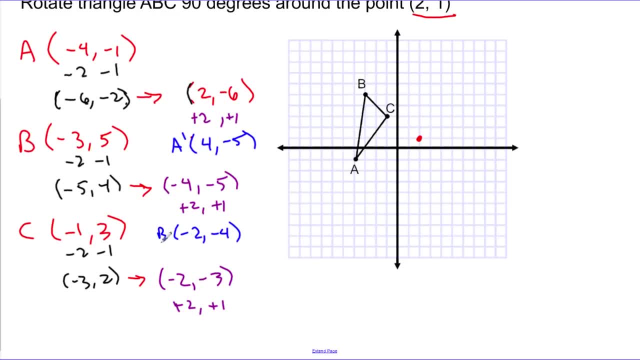 Okay, And I'll call this one b prime finally, because I've done my rotation, okay, And then my c prime I'm going to call it looks like 0, okay, And this looks like negative 2.. So let's plot these points and see what it looks like.